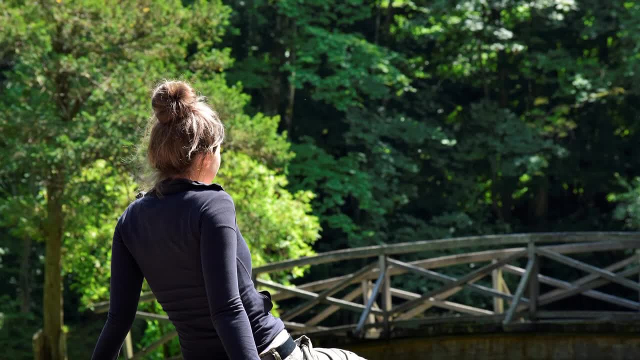 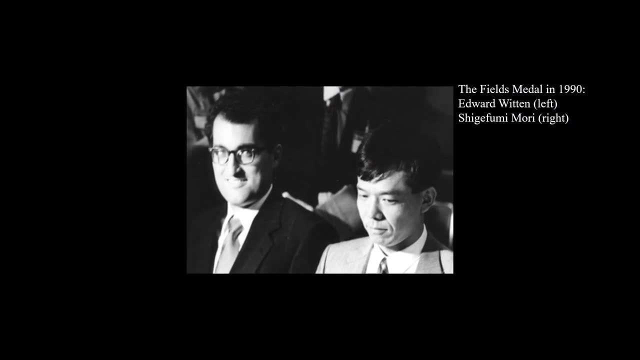 is broken by whatever new heavy scale is broken. The problem is that the mass is not directly equal to the mass of the new heavy scalar field breaks that symmetry. The brilliant mathematical physicist Edward Witten argued in an influential paper in 1981 that supersymmetry had a special 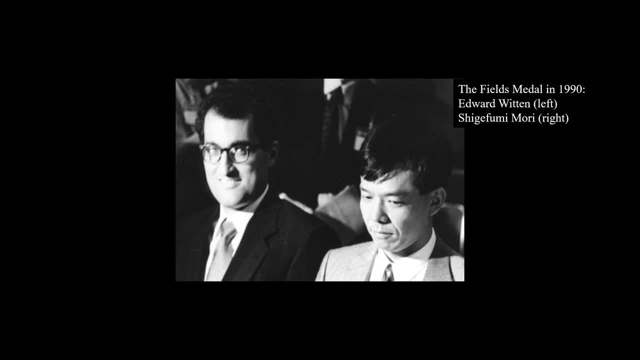 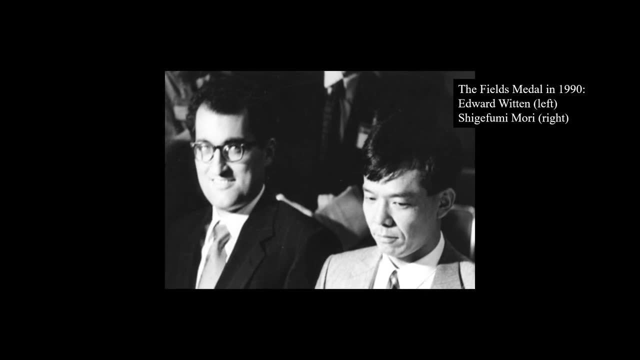 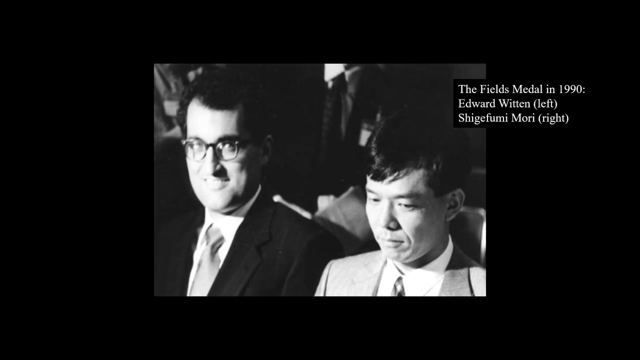 property. It contained the effect that virtual particles of arbitrarily high mass and energy have on the properties of the world at the scales we can currently probe, because virtual fermions and virtual bosons of the same mass produce quantum corrections that are identical except for a sign. If every boson is accompanied by a fermion of equal mass, then the mass of the 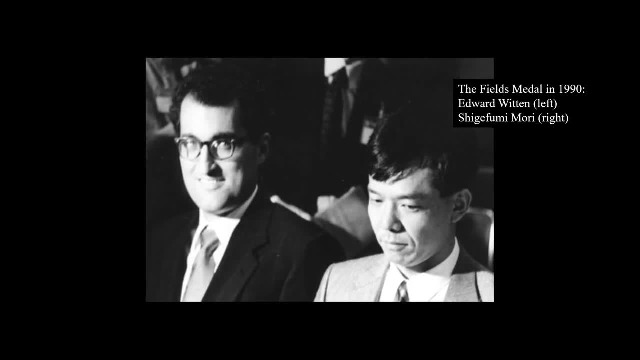 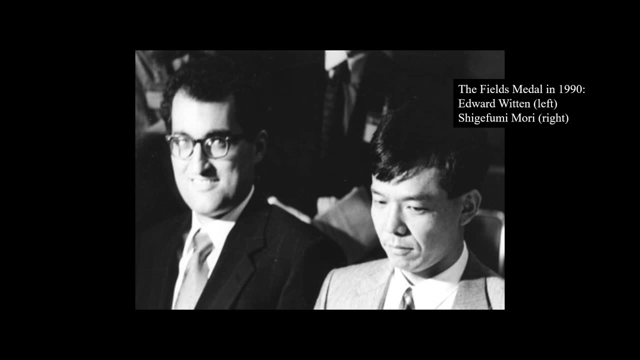 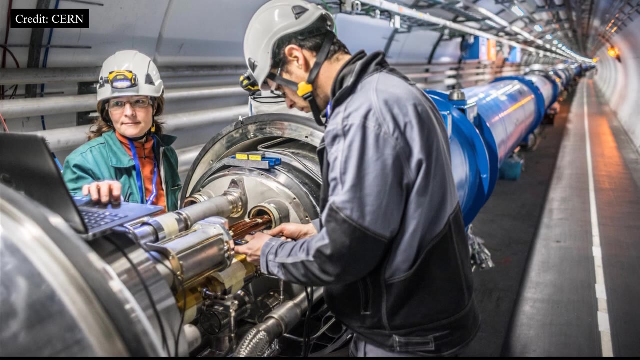 virtual particle is completely broken, This means that the quantum effects of the virtual particles will cancel out. This means that the effects of virtual particles of arbitrarily high mass and energy on the physical properties of the universe on scales we can measure would now be completely removed. If, however, supersymmetry is itself broken, then the quantum corrections 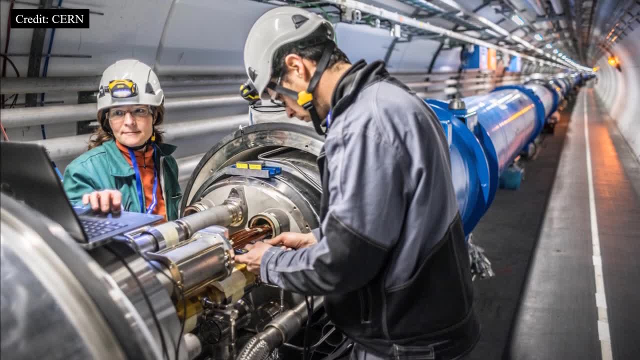 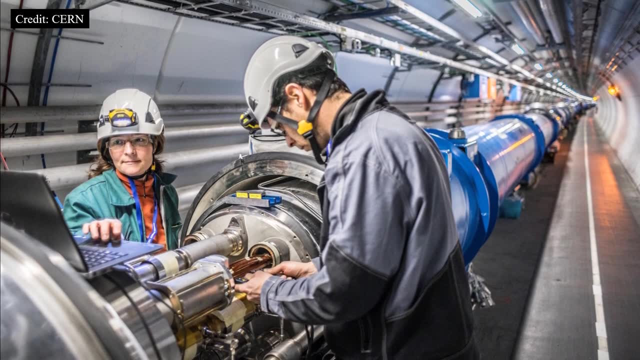 will not quite cancel out. Instead, they would yield contributions to masses that are the same order as the supersymmetry breaking scale. If it was comparable to the scale of the electroweak breaking, then it would explain why the Higgs mass scale is what it is, And it also means we. 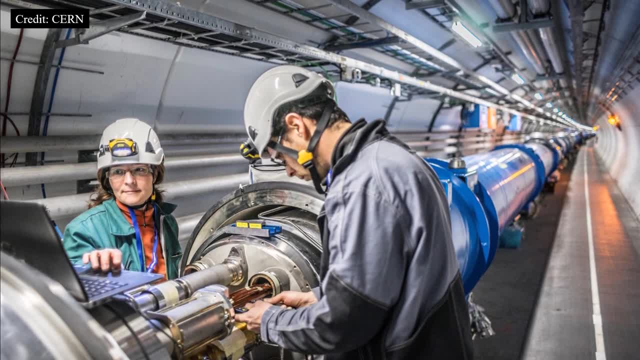 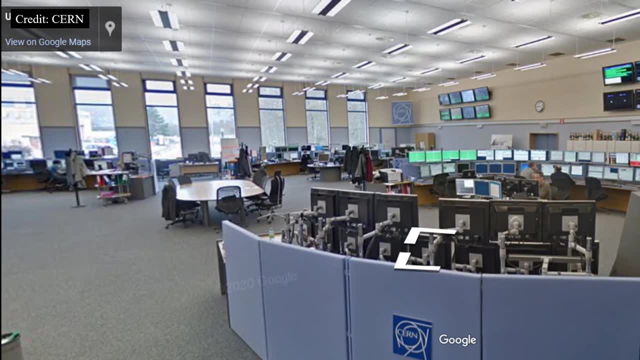 should expect to begin to observe a lot of new particles, the supersymmetric partners of ordinary matter at the scale currently being probed at the LHC. This would solve the naturalness problem because it would protect the Higgs boson masses from possible quantum corrections that 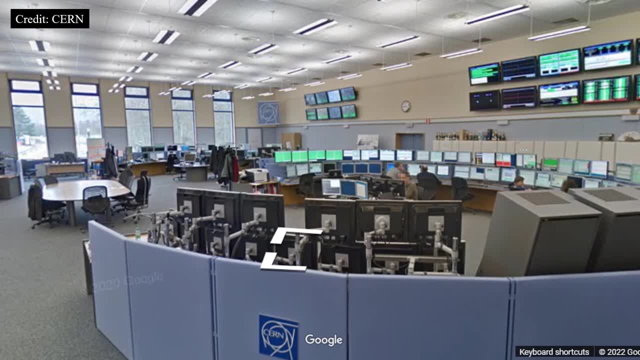 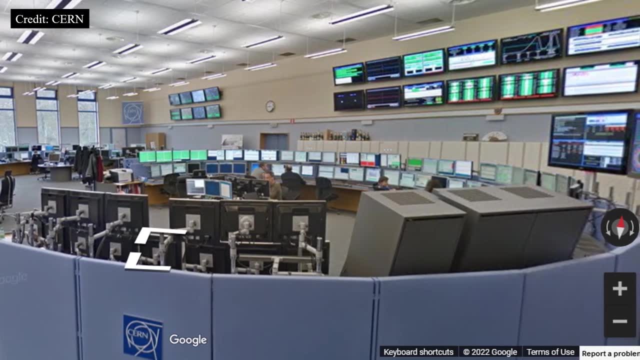 could drive them up to be as large as the energy scale associated with grand unification. Supersymmetry could allow a natural large hierarchy in energy and mass, Separating the electroweak scale from the grand unified scale That supersymmetry could in. 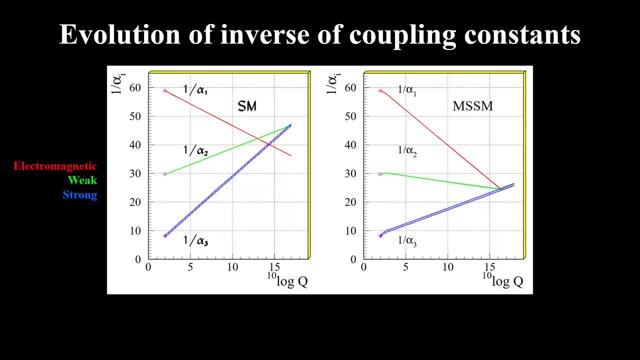 principle solve the hierarchy problem, as it has become known, greatly increased its stock with physicists. It caused theorists to begin to explore realistic models that incorporated supersymmetry breaking and to explore the other physical consequences of this idea. When they did so, the stock price of supersymmetry went through the roof. 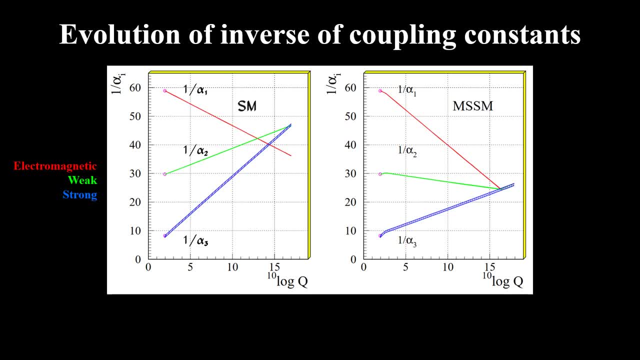 If one included the possibility of spontaneously broken supersymmetry into calculations of how the three non-gravitational forces change with distance, the strength of the three forces would naturally converge at a single, very small distance scale. Grand unification became viable again.